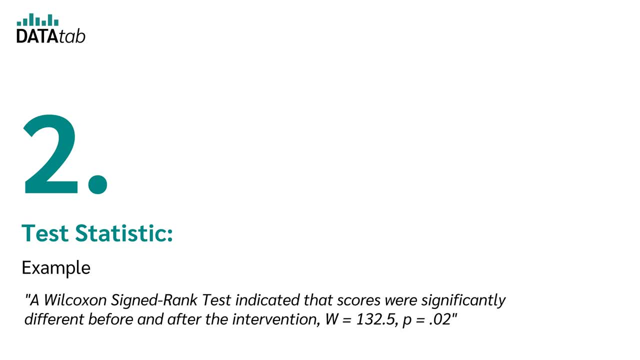 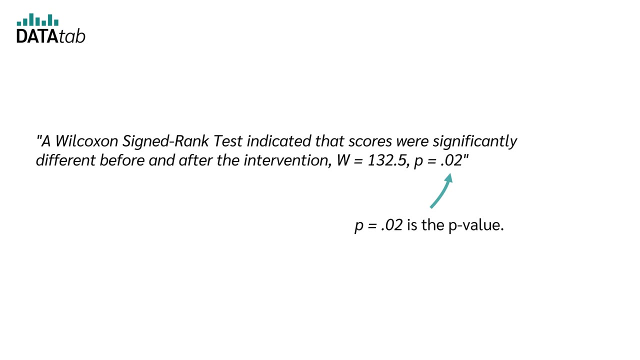 A rank test indicated that scores were significantly different before and after the intervention. w equal to 132.5,. p equal to 0.02.. w is the calculated w-value. p equal to 0.02 is the p-value. Adjust this according to your results. For example, p equal to 0.045,. p equal to 0.25.. 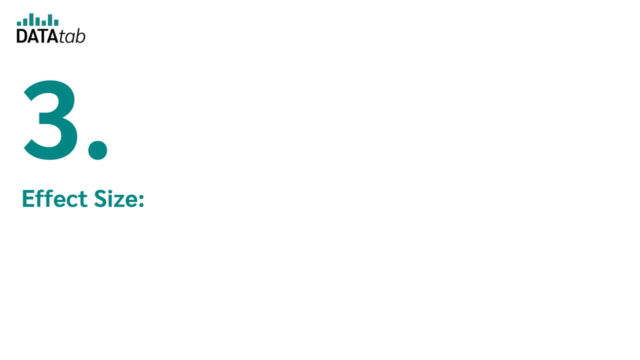 And so on and so forth. Number three: effect size. It's recommended to include an effect size such as r. This provides the reader with an understanding of the magnitude of the difference. The effect size r for the Wilcoxon test can be calculated as r equal to z divided by the root of. 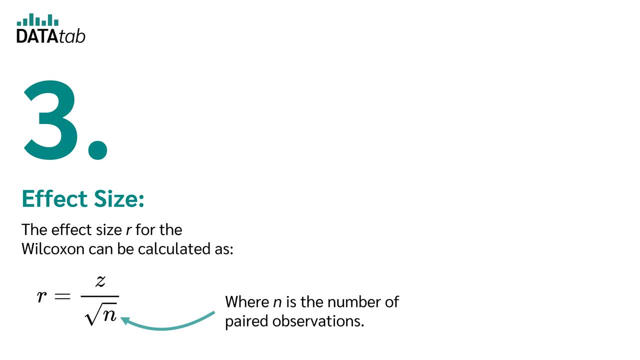 n, where n is the number of paired observations. Example: the effect size was modulated by the number of paired observations. For example, the effect size was modulated by the r equal to 0.40.. For the interpretation of the effect size, you can use this table. 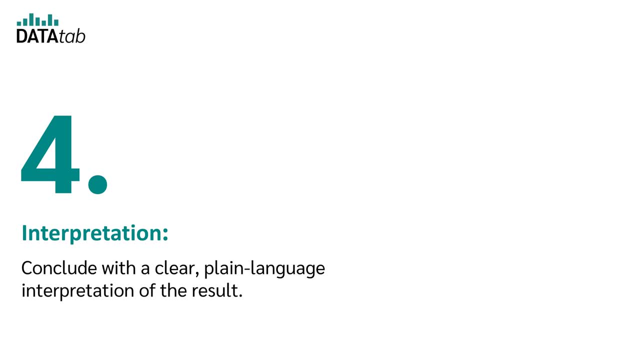 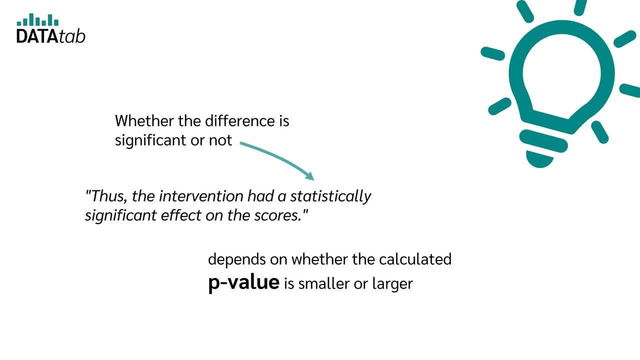 Number four: interpretation. Conclude with a clear plain language interpretation of the results Example: does the intervention have a statistically significant effect on the scores? Whether the difference is significant or not depends on whether the calculated p-value is smaller or larger. 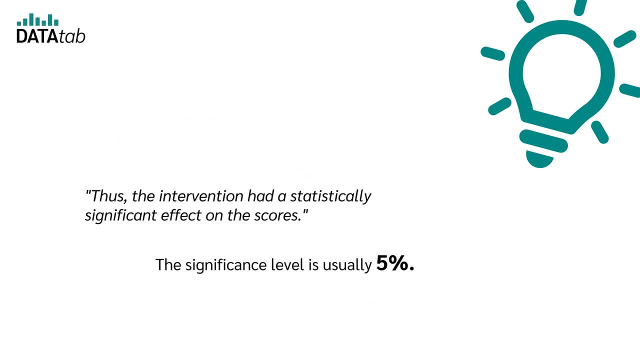 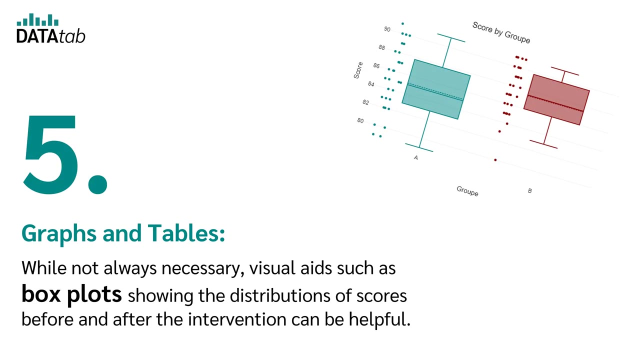 Number five: graphs and tables. While not always necessary, visual aids such as box plots showing the distributions of scores before and after the intervention can be helpful. Ensure that any visual aids are not too large or too small. If the p-value is less than 0.05, there is a significant difference. 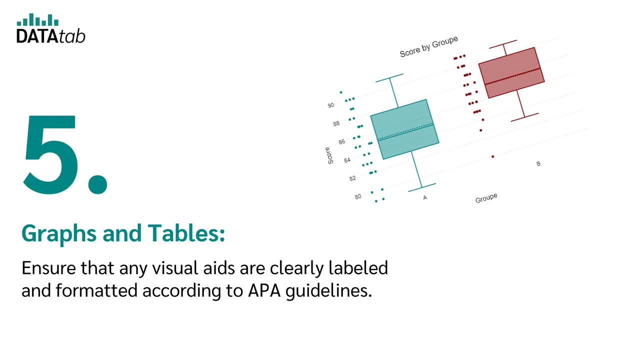 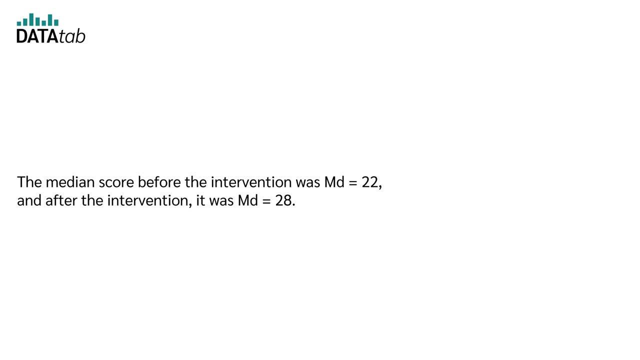 Here is a complete example. The median score before the intervention was md equal to 22 and after the intervention it was md equal to 28.. A Wilcoxon-signed rank test indicated that scores were significantly different before and after the intervention: W equal to 132.5,. p smaller than 0.05,.